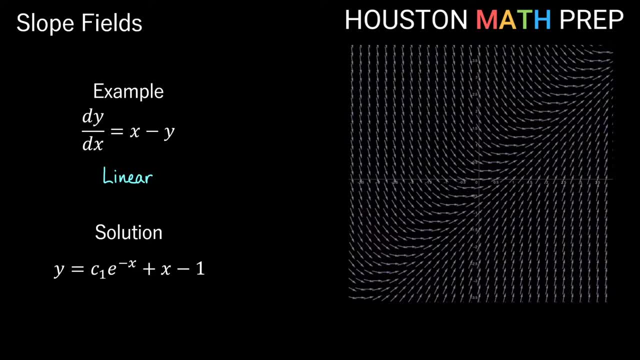 If we look at the slope field you can see that basically from both directions directions- all of the slopes are kind of swooping into one diagonal line here. We call this diagonal line an isocline, So that's basically a region, this line here where all of the slopes are the 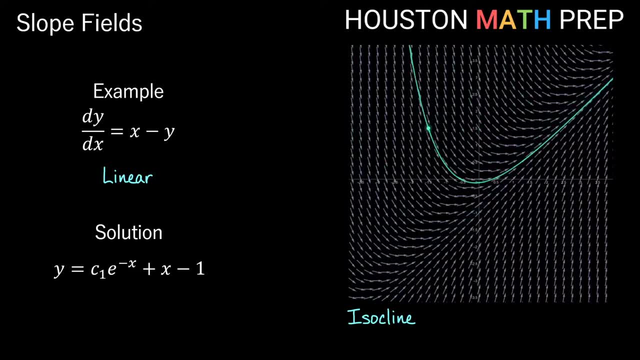 same. If I started on that line as an initial condition, I would stay on that line. But if I am one side of the line, I will swoop in toward that line from one side. If I'm on the other side as an initial condition, I will swoop in closer and closer toward that line. the isocline from: 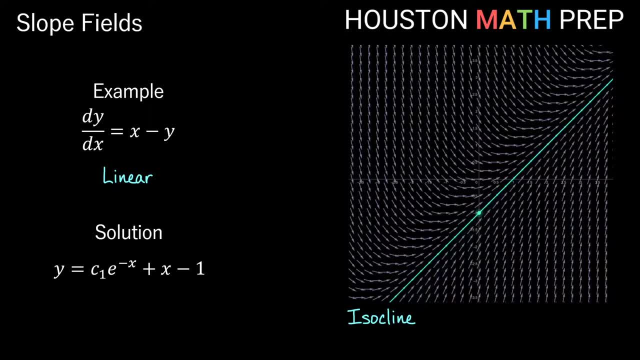 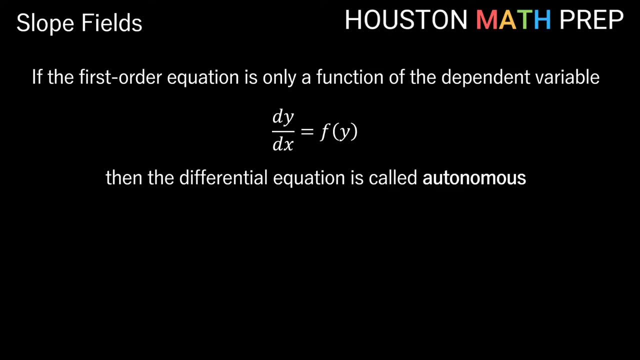 the other direction. So that's the idea of an isocline in a slope field. If our first-order differential equation is just a function that only involves y, the dependent variable, so our right side is an expression that only involves y, then our differential equation is actually referred to. 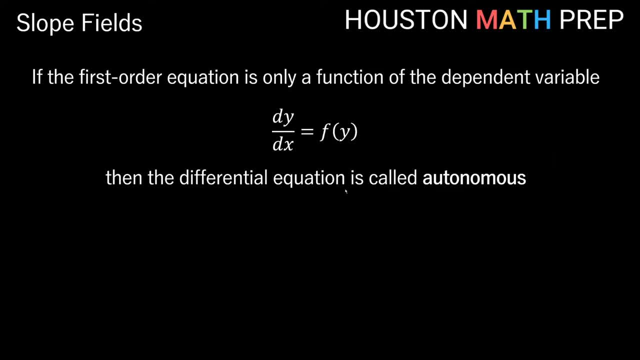 as autonomous when we're thinking of dependent versus independent variables. So when I see the statement dy- dx here- y is a function of x- that tells me y is the dependent variable and x is the independent variable. So in an autonomous equation that's dy- dx equals, we wouldn't have any x variable on the right hand. 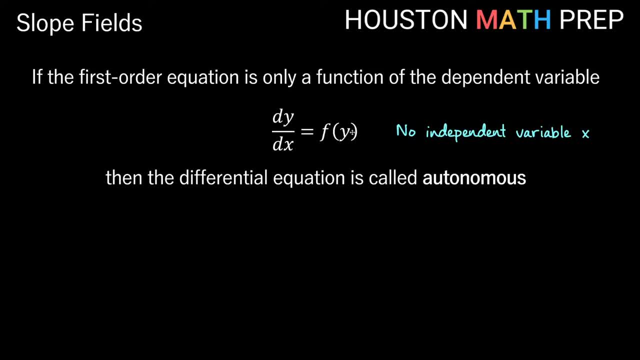 side. If this is true and we're actually able to set our right hand side equal to zero and get solutions for y, then we say that the differential equation has critical or equilibrium points for any value that makes the right hand side zero. In your calculus journeys before this you might have thought as critical. 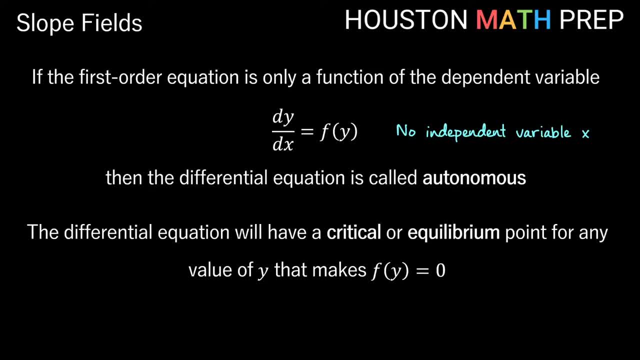 points as x values horizontally, where you found some sort of max or min using a derivative test possibly- And here we just want to make a note that when we're talking about these autonomous differential equations, these will actually be y values, so we'll be thinking vertically in terms of our 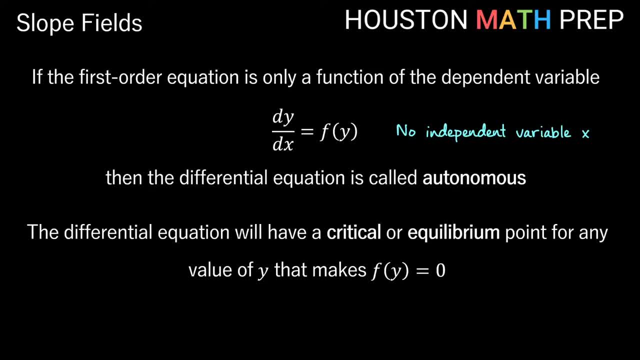 critical or equilibrium points. So if we get some value- let's say y equals C- as our critical or equilibrium point, then basically these critical points are going to give us a constant solution for our differential equation. And when we look at the slope field we'll actually see an isocline, that is, a horizontal. 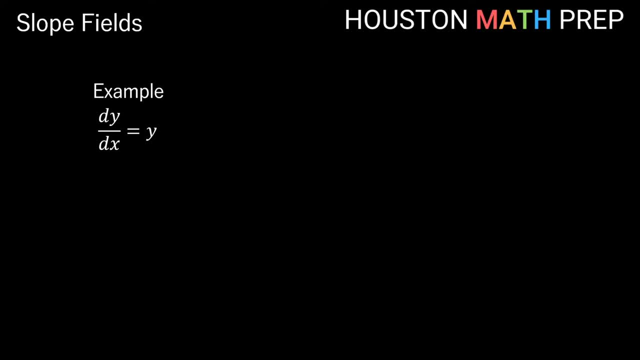 line at those values. Let's look at an example here. we've got this: dy dx equal to y. so you can see, our right hand side is only in terms of y. so this is an autonomous equation. This is also a separable equation. if we were 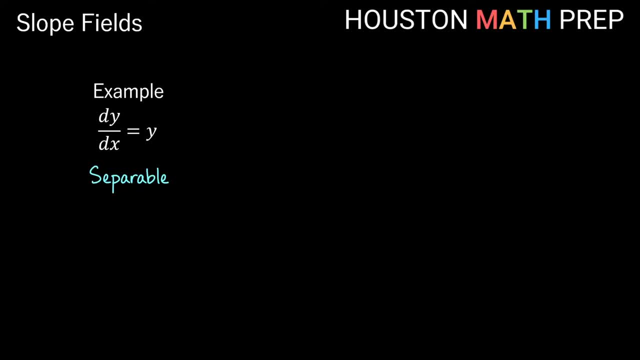 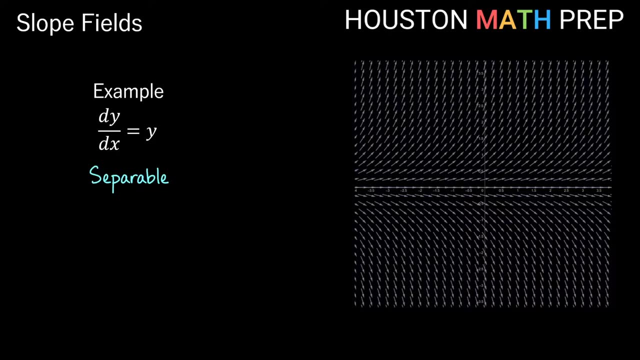 going to solve this using methods by hand, And this is a differential equation that actually gives us the behavior of exponential change. So if we look at the slope field here and I plot some initial condition, you'll see that we get a graph that looks very much like exponential growth here. If I move it to the other, 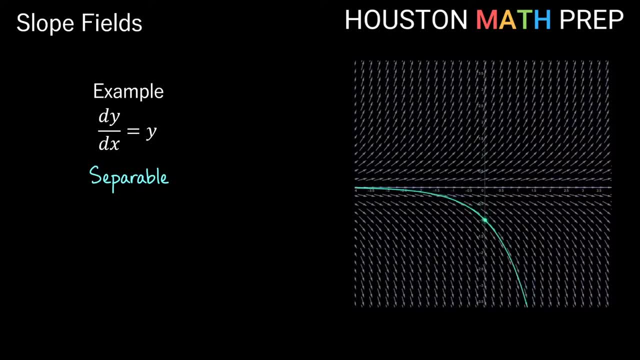 side of the axis, you'll see that we get something that looks like something exponential decline there. So, if we look at our solution, y equals some constant multiple of e to the x, whether that's positive or negative, above or below the axis, If you notice. obviously setting this right side equal to zero and 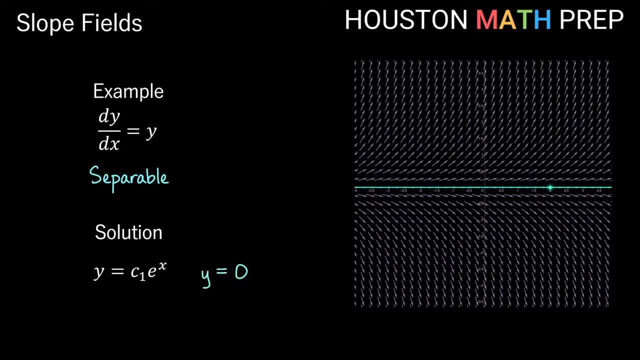 solving. there's not really much to solve. you would just get that y equals zero, and so y equals zero is actually a constant solution. We would call y equals zero an equilibrium point for the differential equation. Looking at another example, here we actually have the differential equation for logistic growth. It would 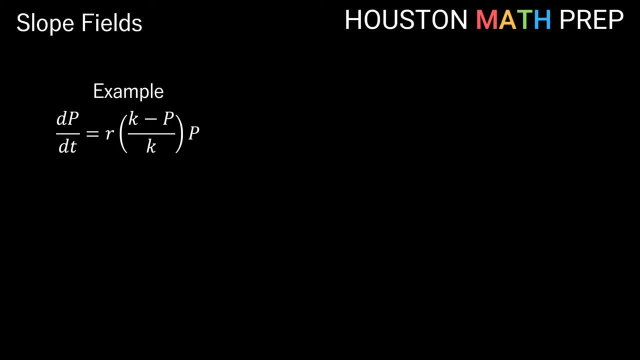 be a little bit difficult to see that this is autonomous in terms of p and t If we swap it over to y's and x's and we notice that r and k are just constants. there is no x term on the right hand side, only y term. so you can see that. 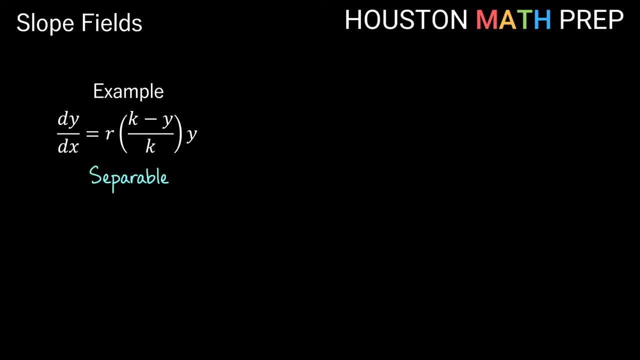 this is an autonomous equation. This equation was actually a separable differential equation and when we solved this equation, we got a solution that looks like this: r was some sort of a rate and, remember, k was what we called the carrying capacity, The max value that we could achieve using this solution. If 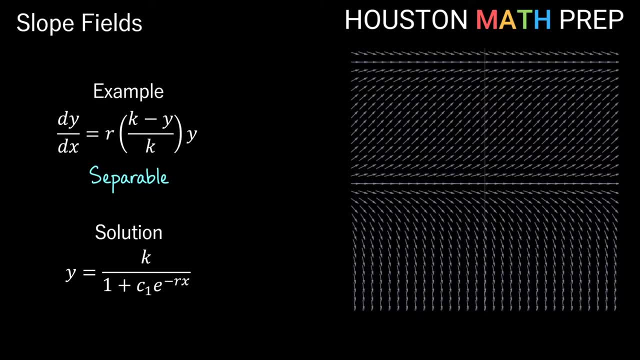 we look at the slope field for this differential equation and we plot some initial condition. you'll notice we get a logistic growth curve. We have some initial condition, some value starting low. it gets higher towards some carrying capacity. We have constant solutions for our differential equation. We have y. 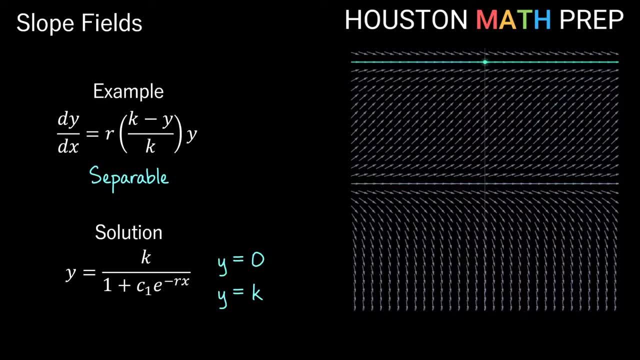 equals zero and actually y equals k the carrying capacity. If we started on either of those lines as an initial condition, we would stay on those lines. If I start between y equals zero and y equals k- our critical points there- then you can see that we're tending upward toward the carrying. 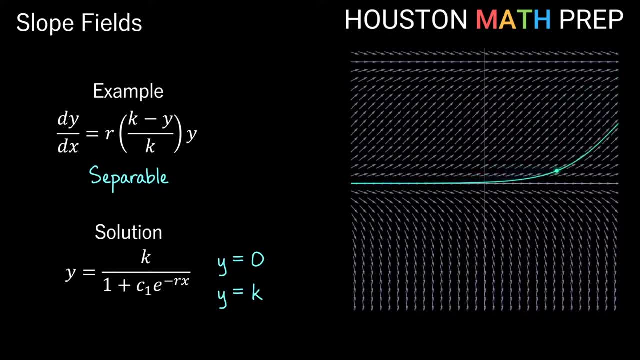 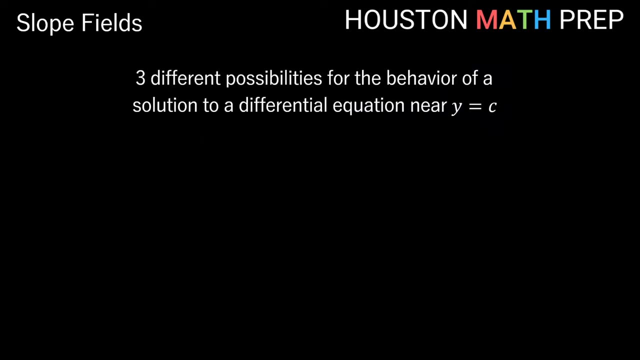 capacity. If we alter the initial condition or we're able to change some behavior of the population, then we can certainly affect the growth significantly as we move horizontally to the right. This is the idea that people mentioned recently about flattening curves when talking about infection rates. If we look at some critical point or 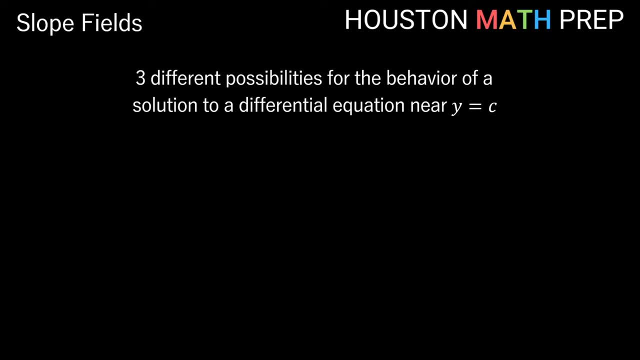 equilibrium point, we look at the constant solution. at that point there are three different possibilities for the behavior of a solution near that constant solution. One possibility for our solution is that it's asymptotically stable, which is what we call an attractor- The idea that if I start on some solution that is near this constant, 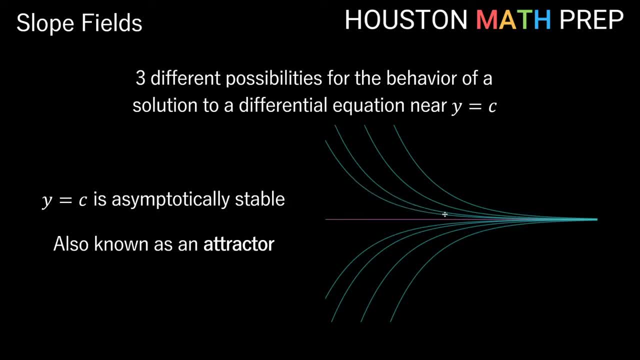 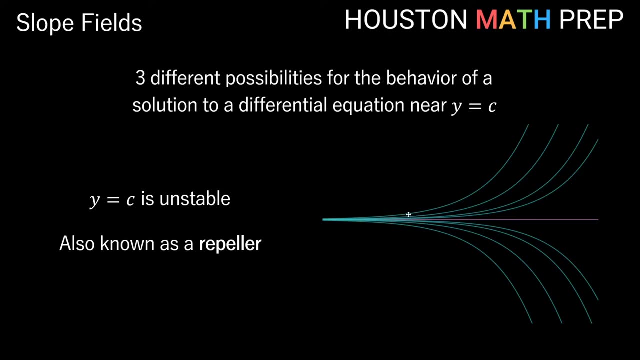 solution and I travel horizontally to the right on my solution curve, I actually will get asymptotically close to this attractor. this y equals some constant. here We can also have some y equals c- some constant solution. that is unstable. If I have some solution curve and an initial condition that is near 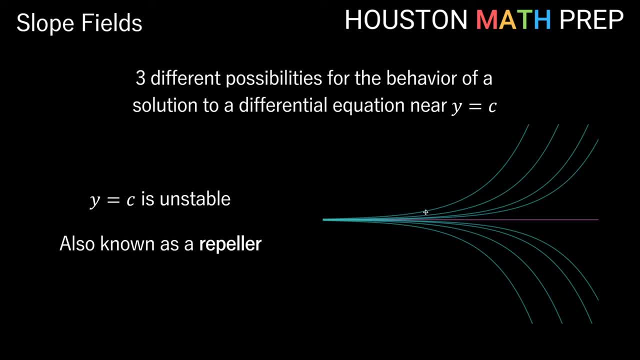 this constant solution and I travel to the right, then I am actually pushed away from this constant solution That is actually called a repeller, in this case opposite of an attractor, And the last possibility is that we have a mixture of both behaviors On one side of the constant solution. I 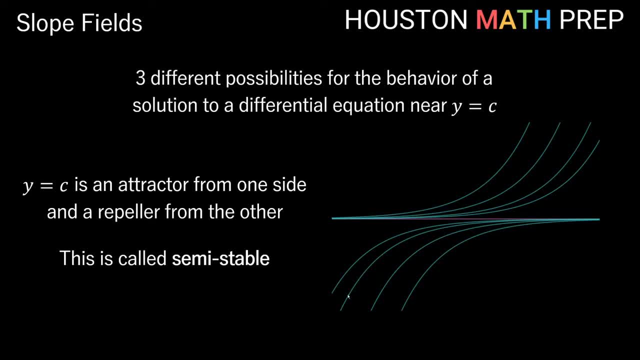 may be repelled from the constant solution as I move to the right and, on the other side, as I move to the right on a solution curve, I may be attracted to the constant solution. We call this a semi-stable solution. We'll look at a couple more autonomous, different. 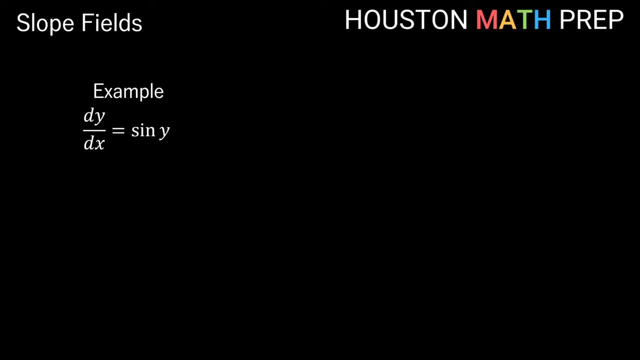 equations and see if we can determine the stability of the constant solutions for them. So here I have dy. dx is equal to sine of y. This is a separable equation and it has a solution that may not look super familiar to you. The behavior of the solutions in particular parts of the xy-plane actually look very. 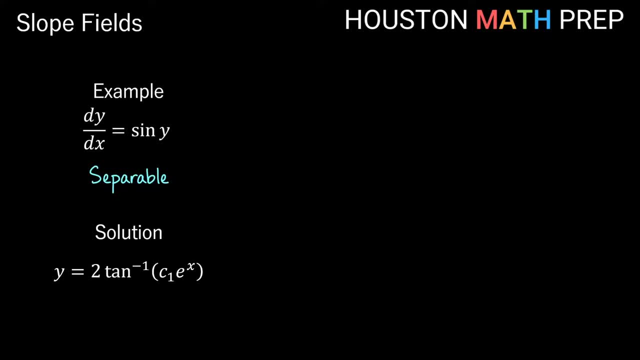 similar to the logistic growth equation that we just looked at. If we think about setting this right-hand expression equal to zero, you should notice from your trig background that we actually get an infinite number of solutions when we set this equal to zero. When you think about angles that have a 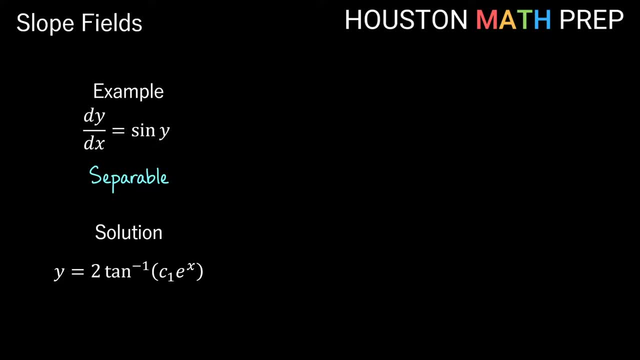 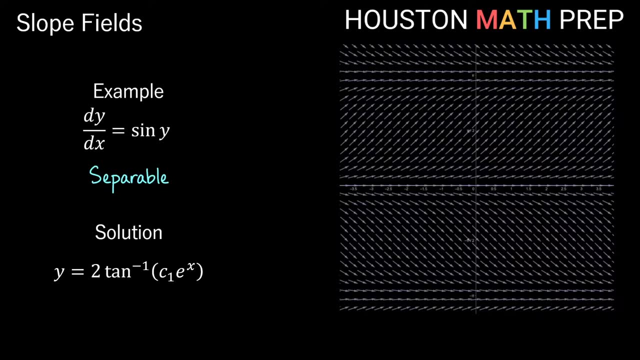 sine value of zero, we will actually get constant solutions every multiple of pi. So if we look at the slope field for this differential equation you can see every pi values vertically we get some sort of a constant solution. So you can see this looks like logistic growth. here We have a constant solution at zero. we 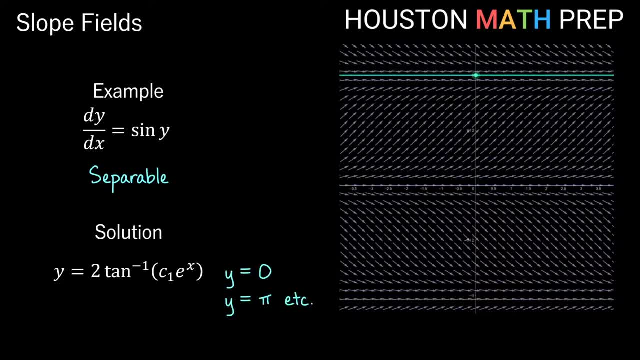 also have a constant solution at pi. We're getting constant solutions every pi. If I look at a condition just below or above, y equals zero. we will have a constant solution at eta: zero. And this: who say we cannot place a constant solution? 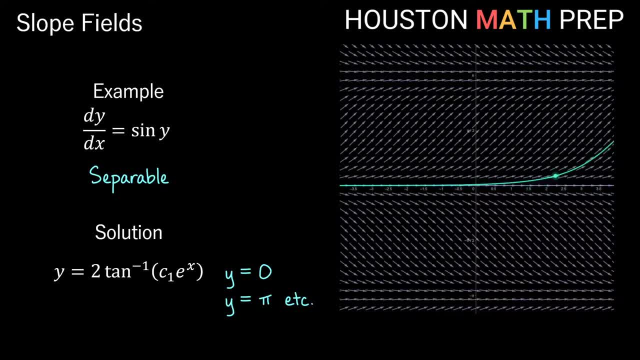 you notice as I travel right on my solution curve, I'm actually heading away from y equals zero. So that means that y equals zero as a constant solution is actually unstable. If you look at y equals pi, you'll notice as I move just. 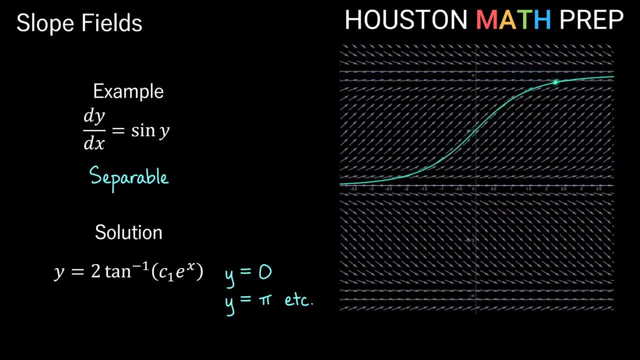 above and below. y equals pi constant solution. as I travel to the right, I'm actually attracted to the value y equals pi, And so y equals pi is actually a stable constant solution for this differential equation, Rather than having to draw an entire slope field to get the general behavior in different horizontal 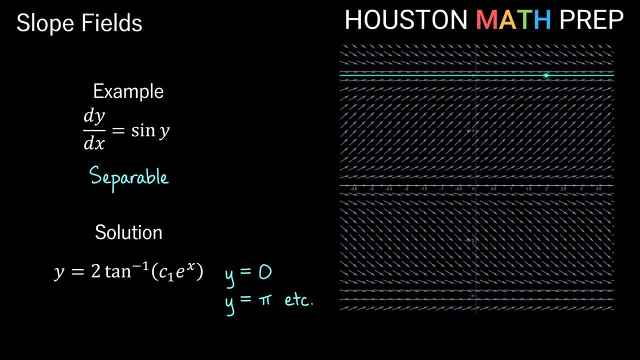 regions of the plane. what we can do is actually draw a phase portrait. This is also called a phase line sometimes. The idea is that we can represent an entire region on one side or another of a constant solution for this differential equation, based on these arrows that point toward or away from the constant. 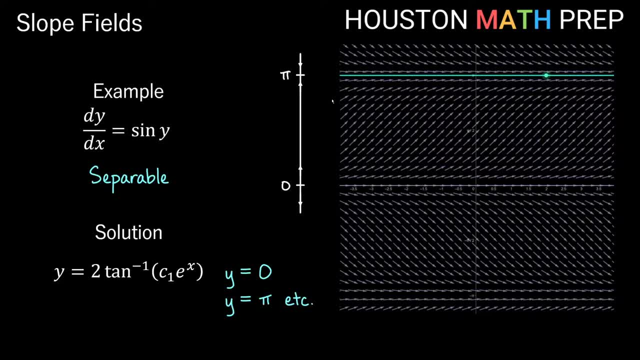 solutions. So here you might notice in between zero and pi as our constant solutions. all of the slopes in between zero and pi are constant solutions. All of the slopes in between zero and pi are constant solutions. All of the slopes in our slope field are going up. We have a positive slope, So you can see that we've 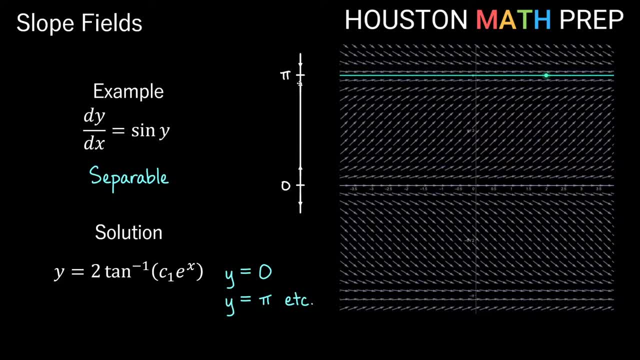 represented between zero and pi. we have little arrows on our phase line that are pointing upward, So we know that the rate of change between zero and pi is positive. You'll also notice that below the axis here we have a negative slope and we've designated that with a downward arrow. A similar thing above y. 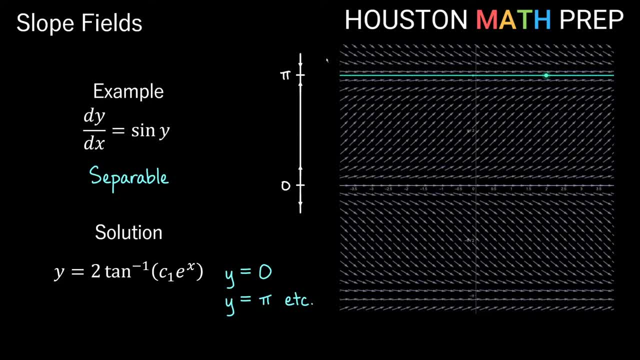 equals pi is our constant solution. You can see that values here we are decreasing toward this constant. so we have this downward arrow as well. These portraits can be convenient to see the stability around a constant solution. So if you look here around, y equals zero. you notice above we're 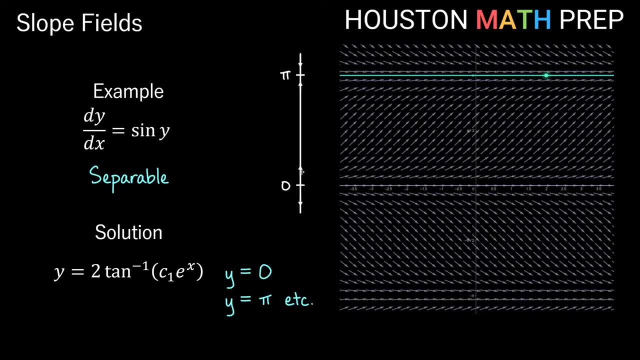 pointing up and below we're pointing down. So this actually indicates that my solutions are moving away from y equals zero. So this would actually be a repeller. If I look around y equals pi, you can see that my arrows are pointing toward y equals pi. So we can see that this constant solution y equals pi is. 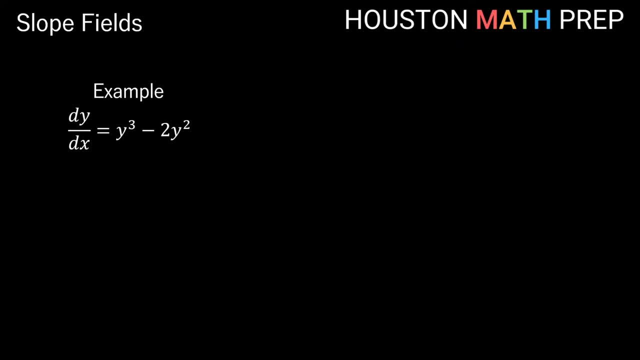 actually an attractor using this phase line. Looking at our last example here, dy dx is equal to y cubed minus 2y squared. So this equation is actually a separable equation. we can separate the variables and solve this. We get an interesting looking general solution as.